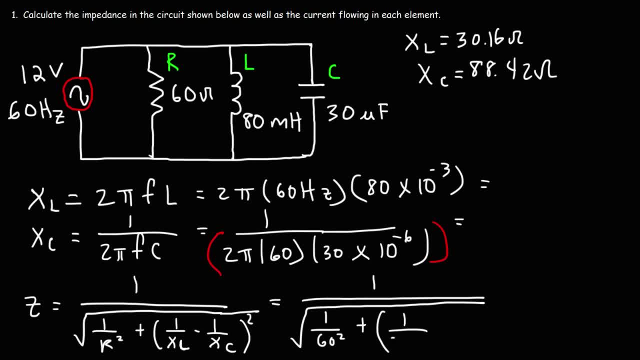 So we have 1 over. let me do that again. So 1 over 30.16 and then minus 1 over the capacitive reactance, which is 88.42.. And then, once you close the parentheses, make sure you square it. 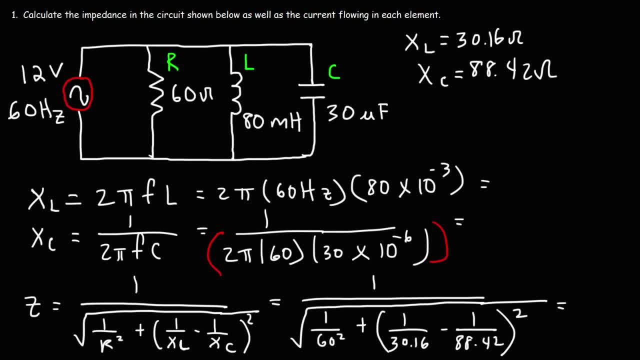 So go ahead and type that into your calculator. You want to be careful the way you type it in. Hold on one second. I'm almost done. So this is the answer that I got for the impedance of the circuit. Okay, impedance is 36.392 ohms, So you can check that as well. Now let's move on to the next part. 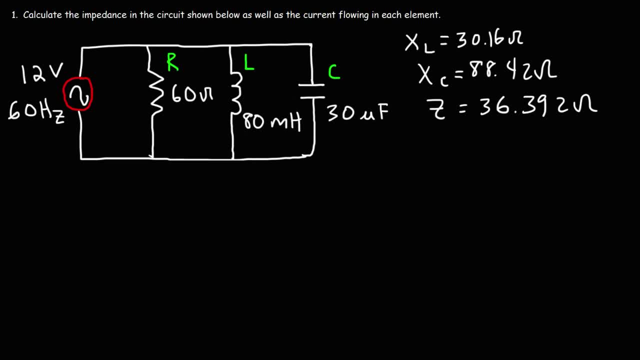 The next thing that we need to do is calculate the current flowing in each element. So let's calculate. the current flowing into the circuit Is: So that's going to be the source voltage divided by the impedance. So the voltage of the source is 12 volts, The impedance of 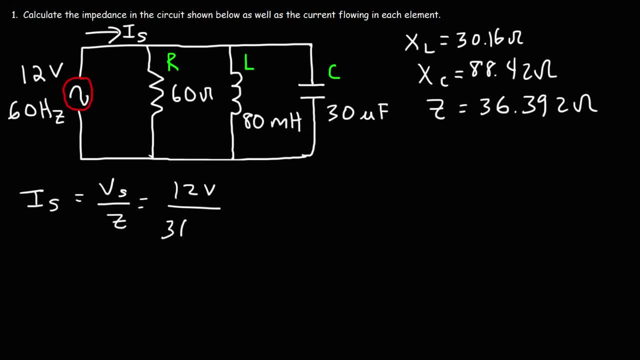 the circuit, we have it right here, that's 36.392 ohms. So dividing those two that's going to be, let's see, 0.32.. 0.3297 amps. So let's write that here: 0.3297.. Now the next current that we need to calculate. 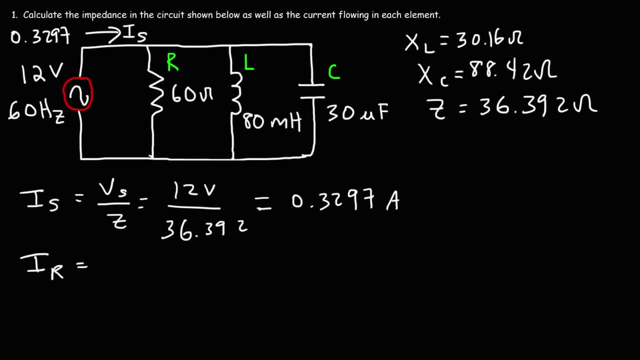 is the current flowing through the resistor, So that's IR. That's going to be equal to the source voltage divided by the resistance. That's based on Ohm's law, So the voltage is 12.. The resistance is 60 ohms. Dividing those two, that's going to be we're going to get. 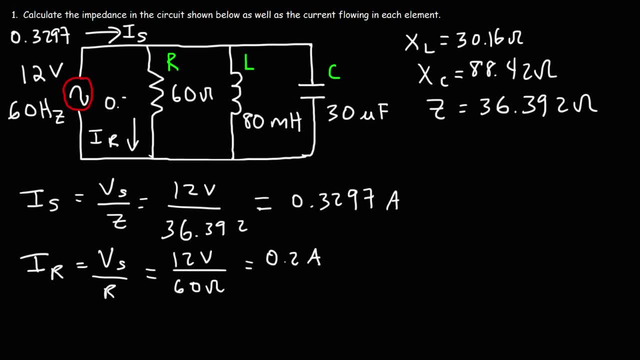 a current of 0.2 amps. So I'm going to put that in the circuit here Now. the next current that we need to calculate is IL, The current flowing through the inductor. So that's going to be VS over XL. 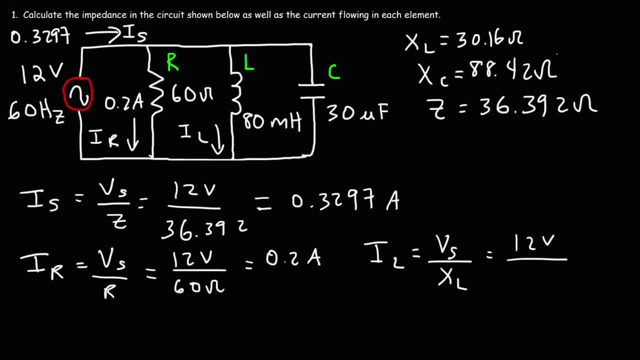 So it's 12 volts. The inductive reactance is 30.16.. So 12 divided by 30.16.. That's going to be- since I'm running out of space, I'm going to put it here- 0.3979 amps, So that's. 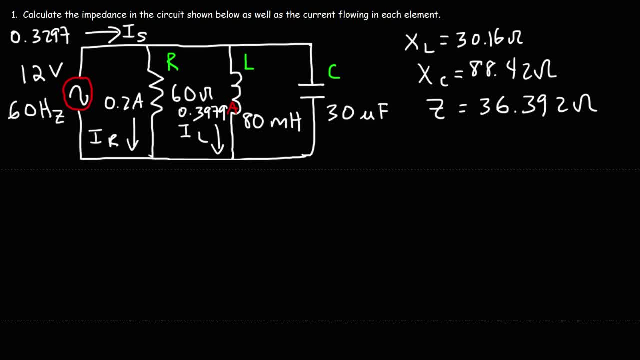 IL. Now there's one more current that we need to calculate, and that is the current flowing through the capacitor, which we'll call IC. So that's going to be VS over the capacitive reactance, And the capacitive reactance is this number here, which is 88.42 ohms. 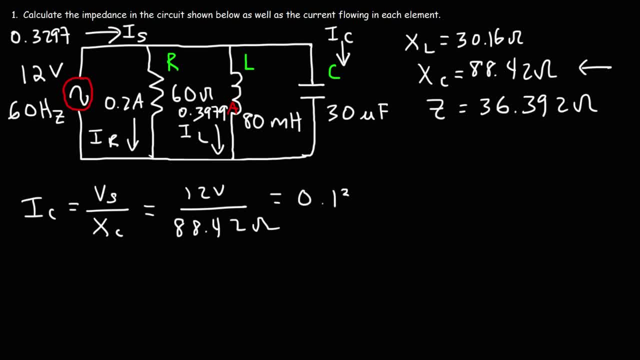 And so we're going to get 0.1357 amps. So now we have the current flowing through each element in the circuit, through the resistor, the inductor and the capacitor. Now notice that IS is not the mathematical sum of IR. 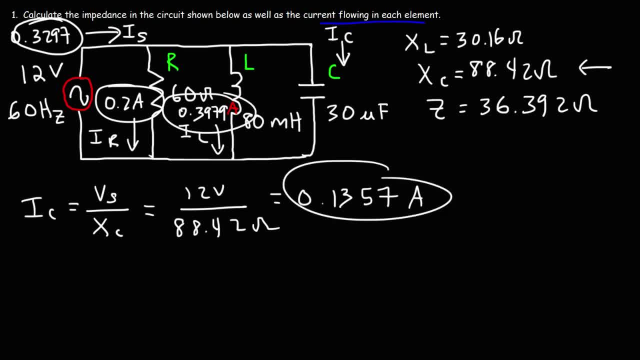 IL and IC. If we were to add up those values, let's see what we'll get: IR plus IL plus IC. So IR is 0.2,, IL is 0.3979, and IC is 0.1357.. 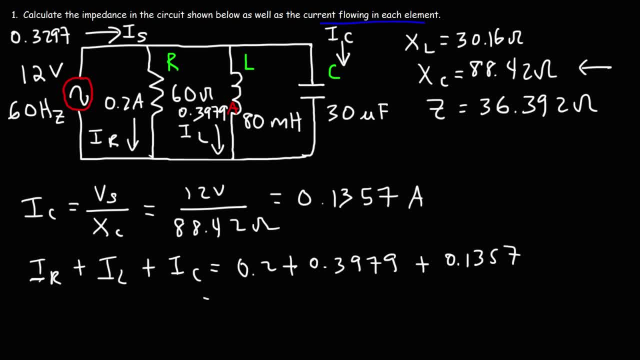 So adding up those values would give you 0.1357.. So that's going to be 0.7336, which doesn't equal IS. Now, even though IS is not the mathematical sum of these currents, it is the vector sum. 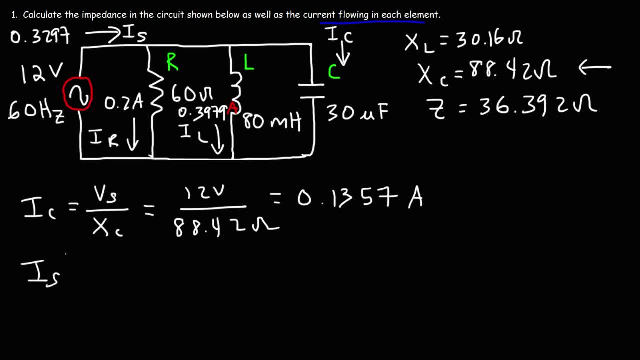 IS squared is equal to IR squared plus IL minus IC squared, So that's going to be 0.7336, which doesn't equal IS. Now, even though IS is not the mathematical sum of these currents, it is the vector sum. So that's going to be 0.7336, which doesn't equal IS. 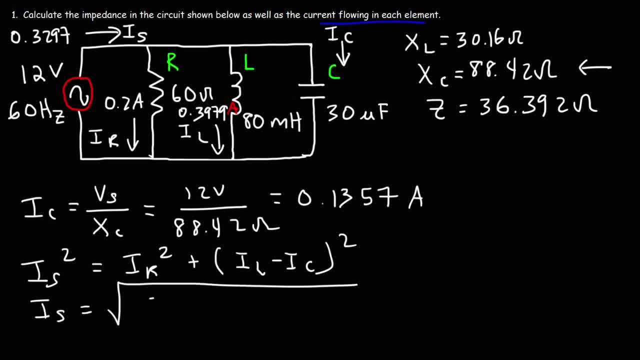 Now, even though IS is not the mathematical sum of these currents, it is the vector sum, So we're going to use this formula to confirm it. This is a good way to check to make sure you have the right answer in this problem. So the current flowing through the resistor is 0.2.